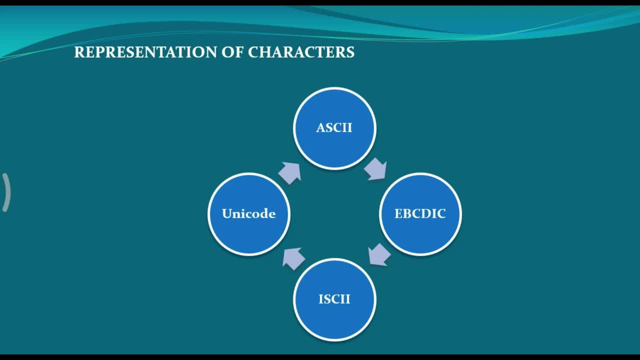 characters in a computer. For representing characters in computer generally we use four codes. First one: ASCII, APSCIDIC, ISCII, UNI code. These are the four character representation codes that I will explain in this video. I have already taught characters are alphabets in languages and special symbols. 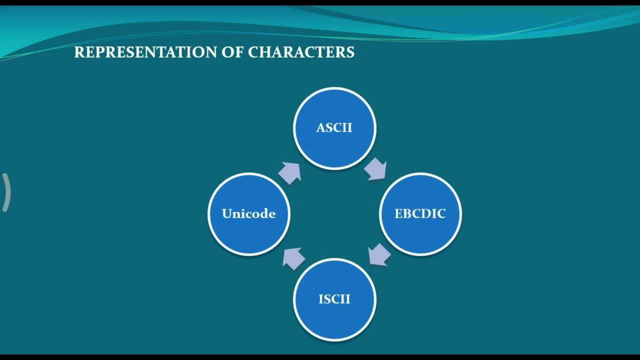 characters are alphabets in language and special symbols: characters are alphabets in language and special symbols: Dot quotation: single quote less than greater than These are the symbols that also include in the characters. First one: ASCII. ASCII stands for American Standard Code for Information Interchange. 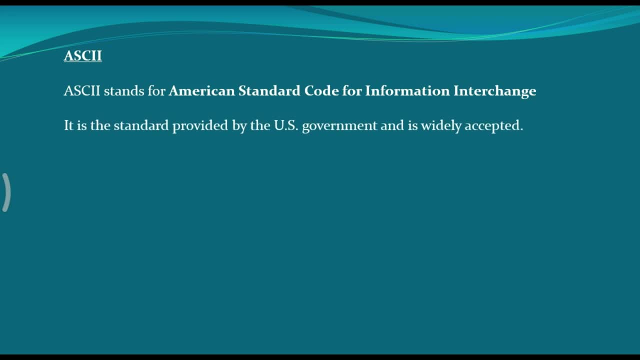 It is the standard provided by the US government. after that it become widely accepted. ASCII is a unique integer number assigned to each character In ASCII code. there are unique numbers for each characters. There are two types of numbers. There are two types of ASCII. 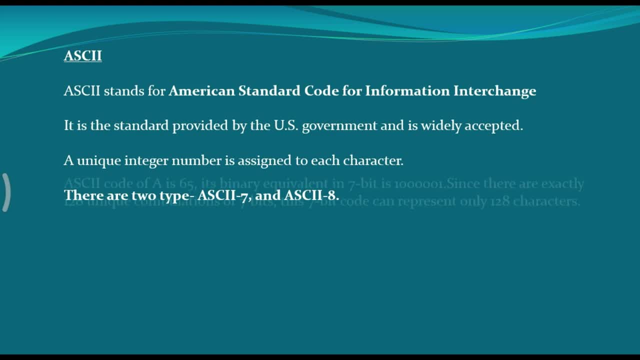 ASCII 7 and ASCII 8.. ASCII code for A65. Its binary equivalent. in ASCII 7 bit is 1000001.. In this binary there are 7 bits, So in ASCII 7, 7 bits are used to represent a character. 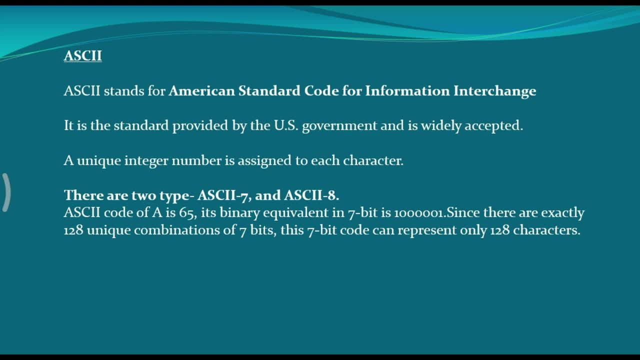 Here I have given one example, that is, the code of A capital letter, A, Capital A in XR, decimal 65.. In binary it is 1000001.. zero one, since there are exactly 128 unique combination of seven bits. so you using seven bits. 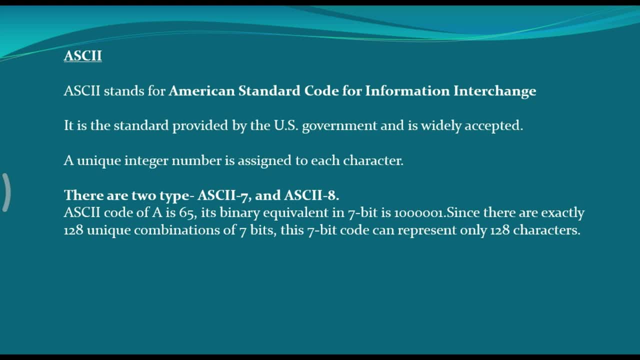 we can represent 128 unique characters. so ask is seven code can represent only 128 characters, because 2 raise to 7 is 128. so but in the case of asky 8, there are 8 bits to represent each characters. so we can represent. 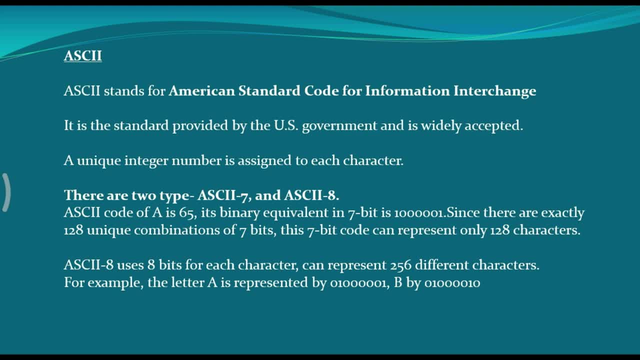 2 raised to 8, that is equal to 256. using ascii 8 we can represent 256 different characters. for example, the letter f, capital letter a, is represented by zero one 0, 0, 0, 0, 0, 1 and B by 0, 1, 0, 0, 0, 0, 1, 0. in ASCII 7. there are only 7 bits in ASCII. 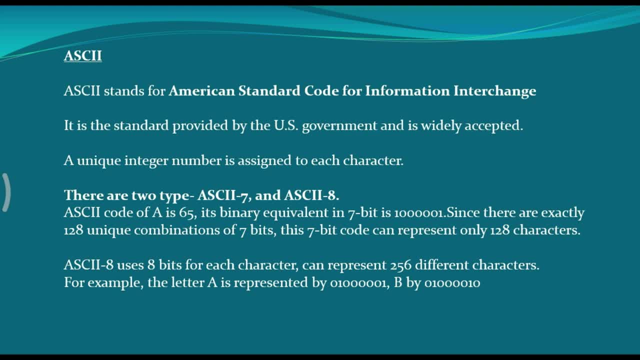 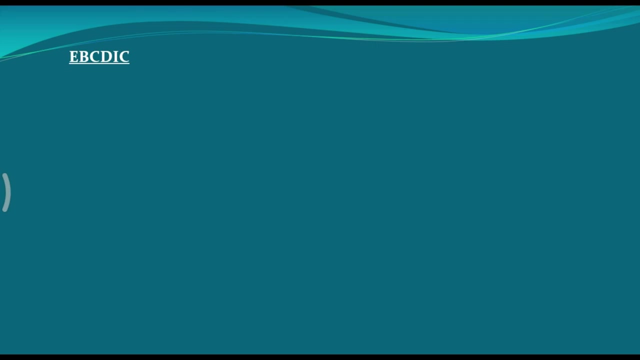 8. there are 8 bits for each characters. using ASCII 7, we can represent maximum 128 characters. using ASCII 8, we can represent maximum 256 different characters. these are the two difference between ASCII 7 and ASCII 8. next, EPSIDIC. EPSIDIC stand for extended binary coded decimal interchange code. it is similar. 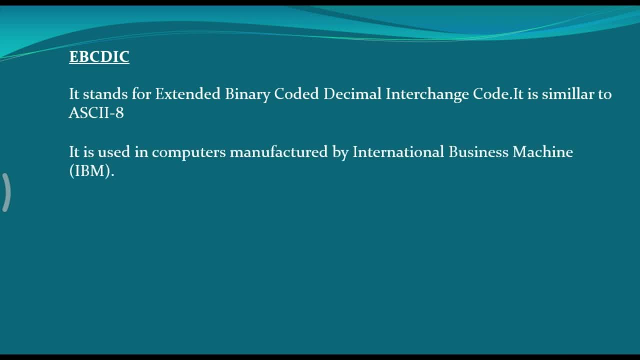 to ASCII 7 and ASCII 8. it is used in computers manufactured by the company international business machines, that is, IBM. it is capable of encoding 256 characters because it uses 8 bits to represent each characters. ASCII codes and EPSIDIC code can be transformed to each other. 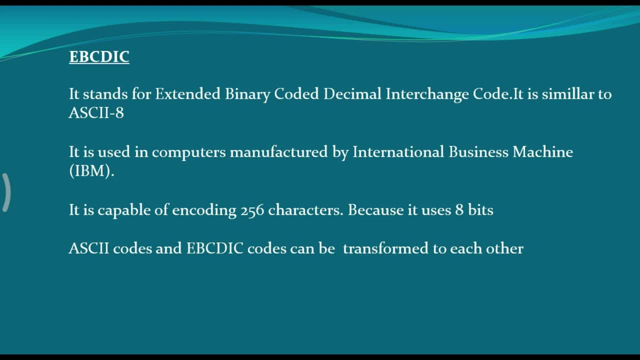 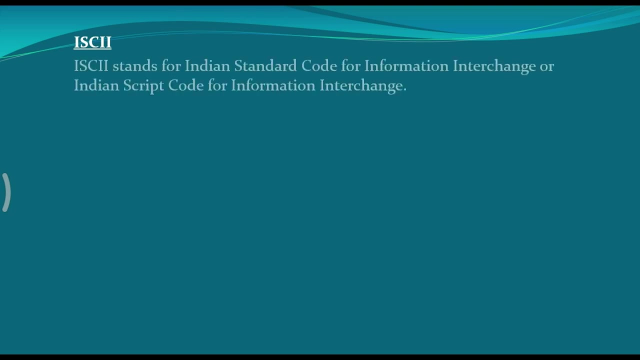 for example, if one computer use ASCII 9 Mb, so we can convert APT Snap sound as to ASCII, we can convert ASCII code to APS decía, so interchange in between ASCII and APS d codes are possible. IAC- IA stand for Indian standard- called for information interchange. 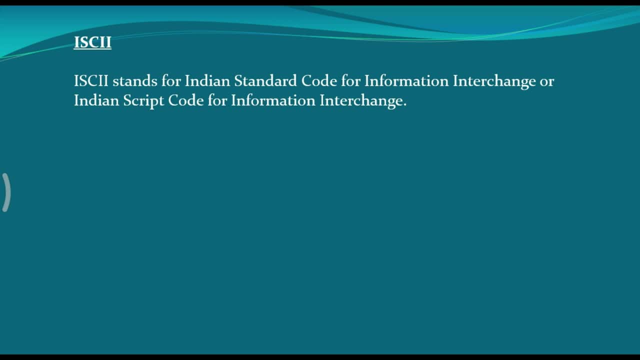 or indian script code for information interchange. it is an encoding scheme for representing various writing system of india, that is, various languages in india. isei uses 8 bits for data representation, so isei use 8 bits to represent each characters. so using isei we can represent maximum 256 characters, that is, 2 raised to 8.. 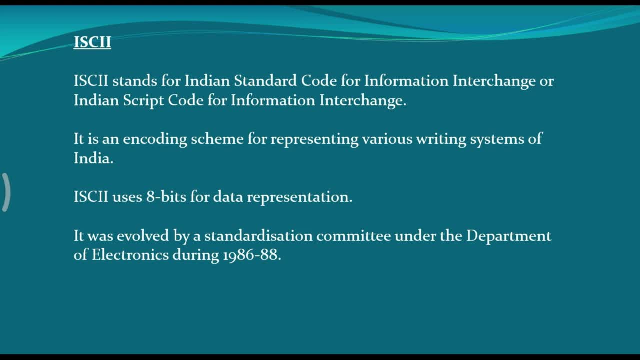 it was developed by a standardization committee under the department of electronics of india government during 1986- 88. now it is adopted by bureau of indian standards and the isei is maintained by bis bureau of indian standard, which is the an organization under india government. 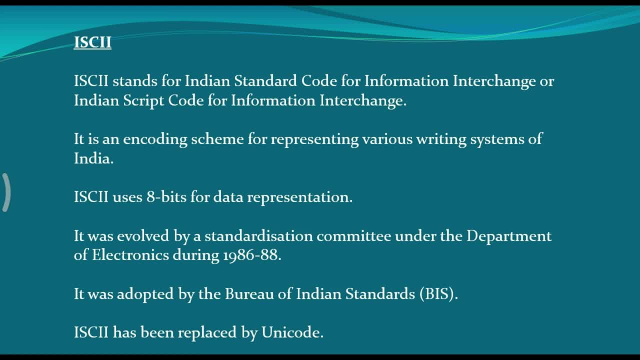 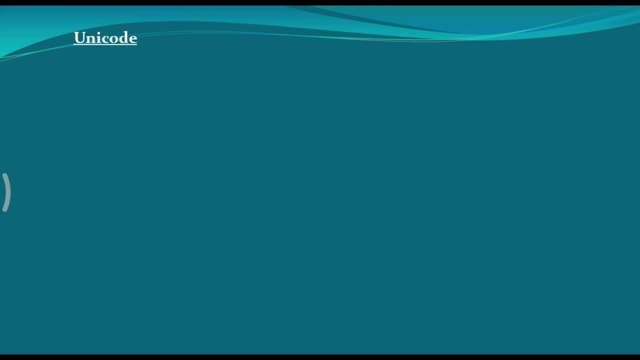 nowadays, isei has been replaced by unique codes that we will explain next. fourth, for the character representation code is unique code, ascii, absidic, and isei uses seven or eight bits which represent 128 to 256 characters only. this cannot represent all characters of written languages of the world. 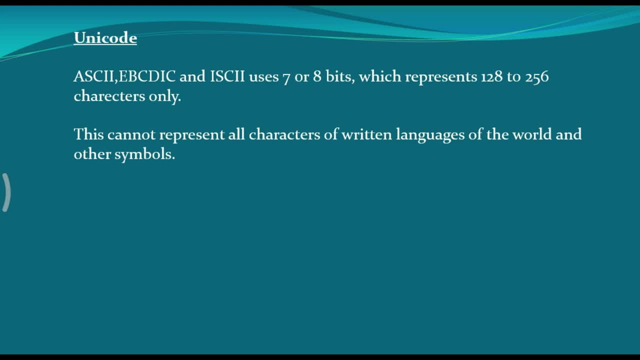 and other symbols. so in the world there are a lot of languages. 256 characters are not not able to represent these different characters in different languages. unicode provide a unique number for each characters, no matter what the and for platform B, so Unicode is used to represent characters or alphabets in.